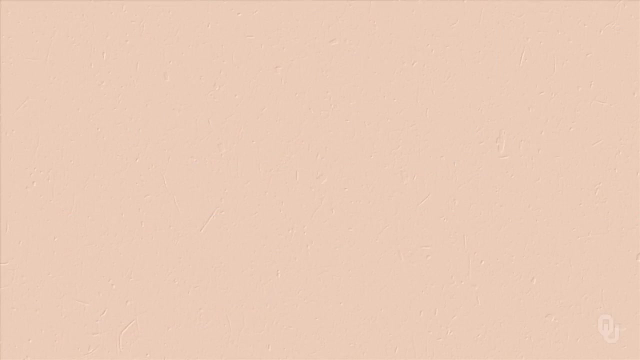 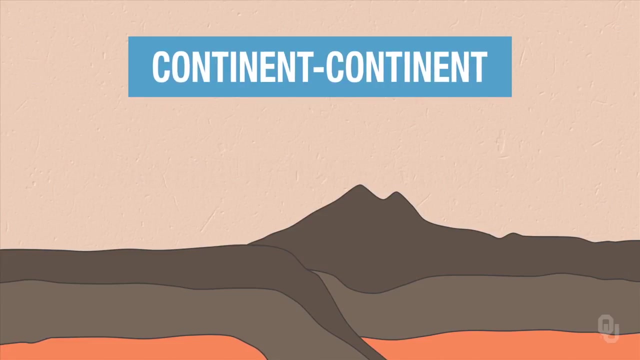 So you get shallow earthquakes. Second type of plate boundary: convergent plate boundary, where plates come together For continent-continent convergent plate boundaries. when two continents collide, what's going to happen? You're going to get mountains, like the Himalayas, You get earthquakes, You get granites And you get faults when the two plates come together. What about at subduction zones, where you have an oceanic plate going, say, underneath a 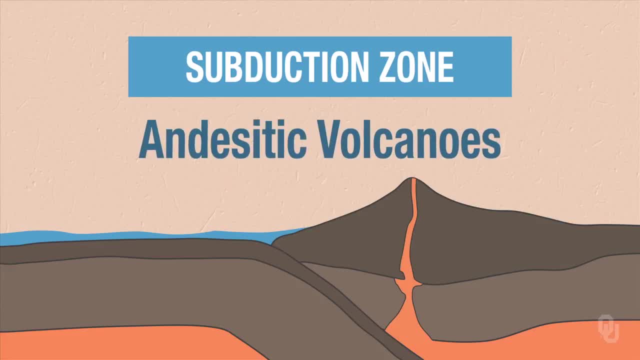 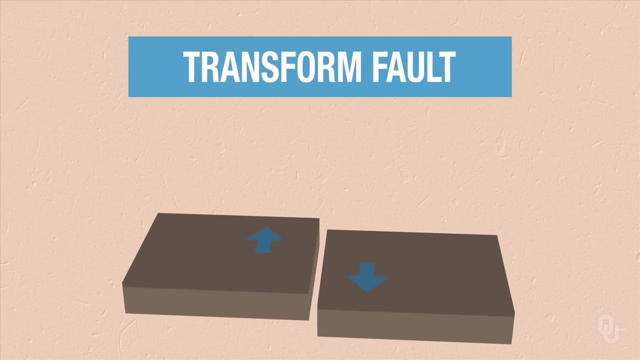 continent. You're going to get volcanic activity and acidic volcanoes which are explosive. You're going to get shallow to very deep earthquakes up to 700 kilometers. And you're also going to get reverse faults, or low-angle reverse faults, called thrust faults, And the third type of plate boundary, the transformed fault boundary. that's where plates move by each other. What happens, Major thing that happens here- will be earthquakes. Think of 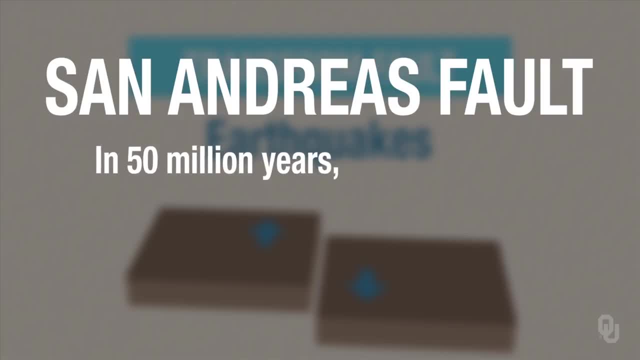 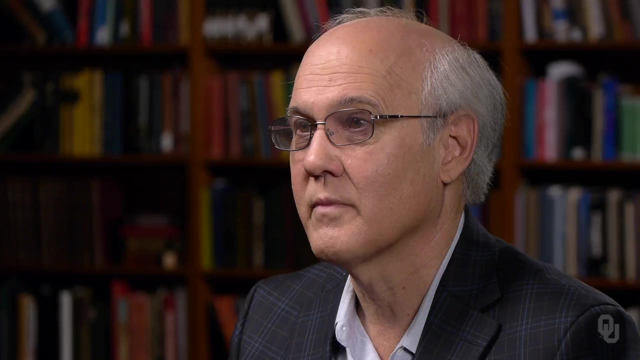 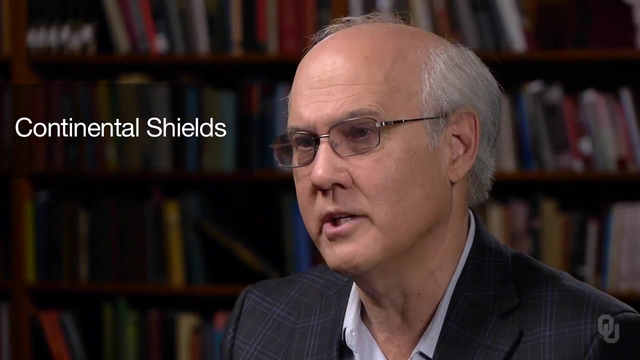 the San Andreas Fault. In 50 million years or so, San Francisco will be due west of LA because of the movement along the San Andreas Fault. Now we will talk about mountain building in more detail as it relates to plate tectonics, But first a little bit more information on the continents. The continents are composed of the continental shields. These are the oldest part of the continents. They're generally pre-Cambrian. 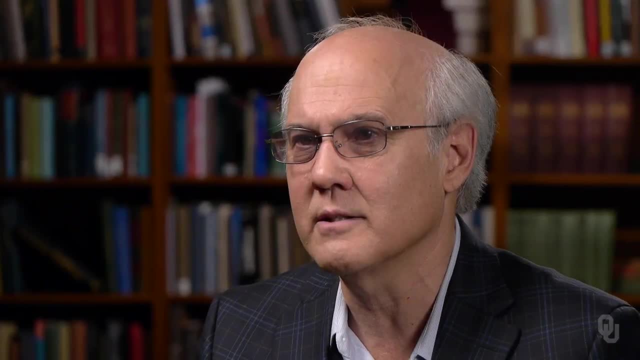 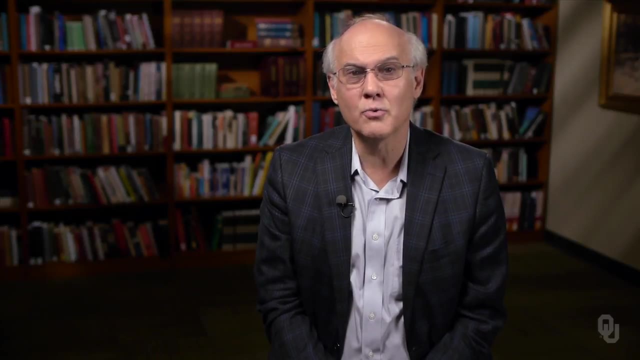 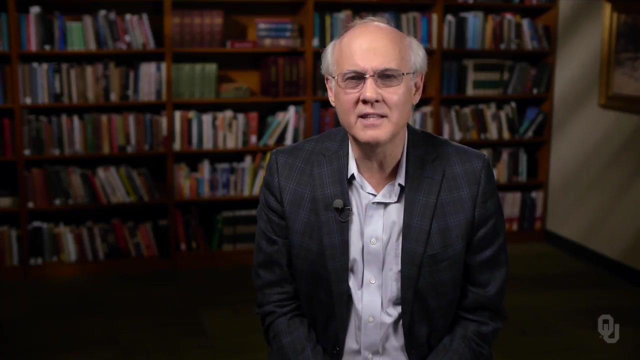 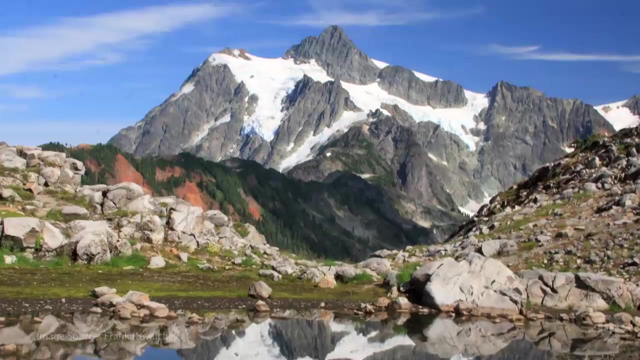 rocks, And they occur in the center part of the continent. In North America they're in what's called the Canadian Shield. These shields are surrounded by younger mountain belts like the Appalachians and the Rockies. So how do we relate these mountains to plate tectonics? Well, some mountains are volcanic mountains, like the Cascades. They occur above subduction zones. The Cascades are in the northwestern United States. The 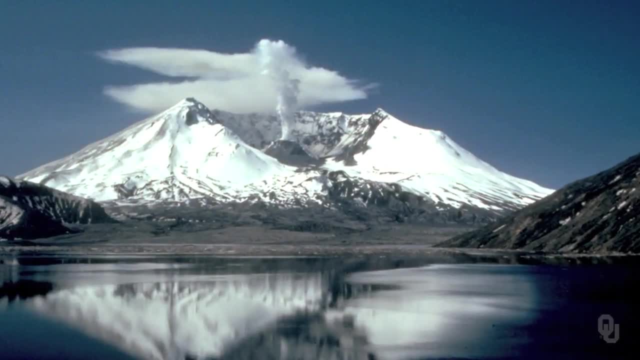 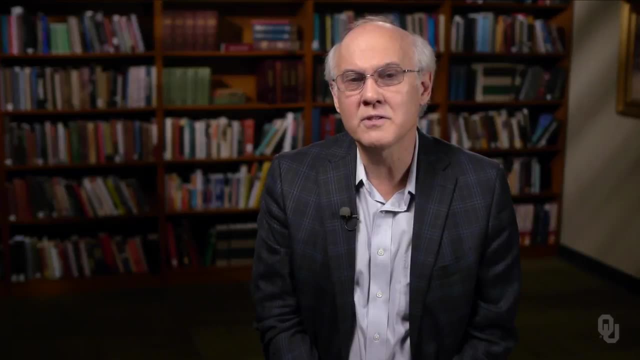 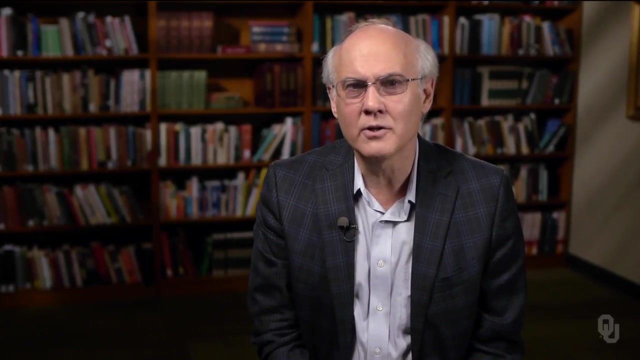 example, volcano, there would be Mount St Helens. We have continent collision mountain belts like the Appalachians and Himalayas. Now there's something very interesting about the relationship between plate tectonics and mountains, and the best way to illustrate that is to think about what's called the